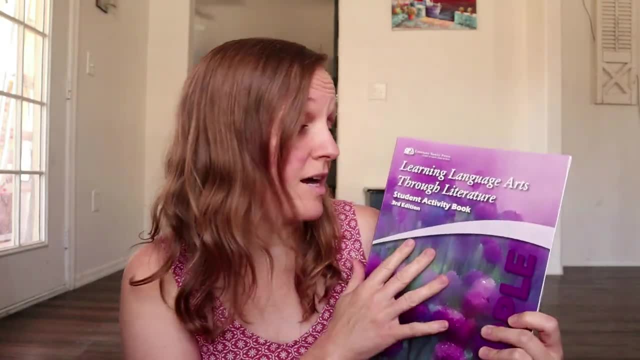 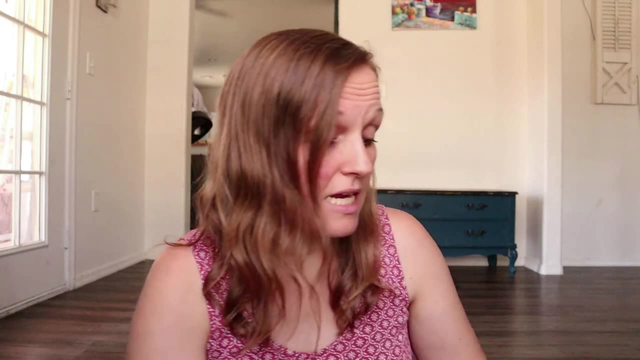 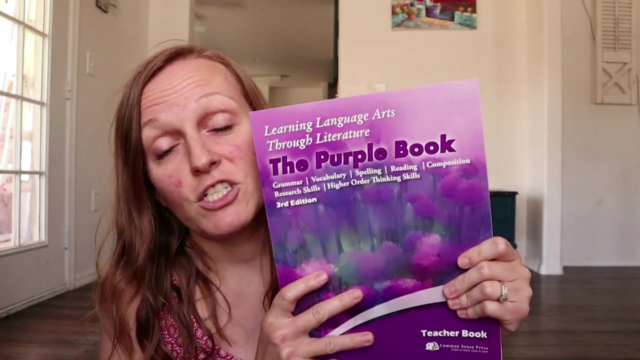 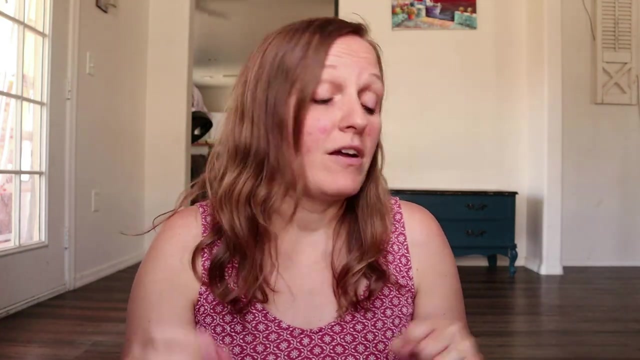 be doing a full flip through through the student guide of Learning Language Arts Through Literature and Language Lessons. for today, I will also give you guys a look inside the teacher's guide for Learning Language Arts Through Literature, and I will have time stamps down below, so if there is one that you want to see in particular, then you can skip ahead. I will also have. 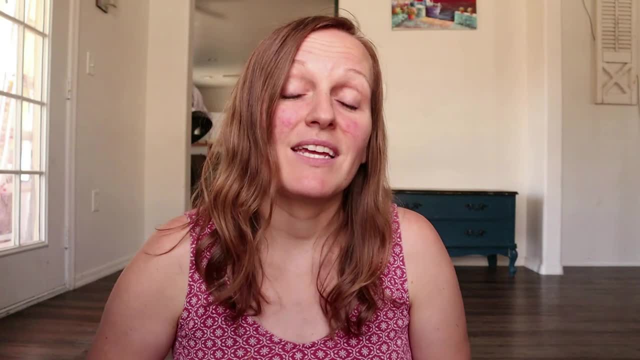 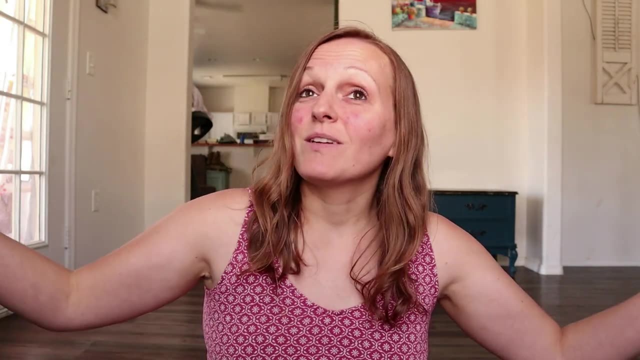 a comparison chart at the end of this video. So I am going to turn around the camera and start that flip through, talk to you guys about it, show you a look inside and hopefully make your- your language arts decision making for this coming year a little bit easier. Alright, you. 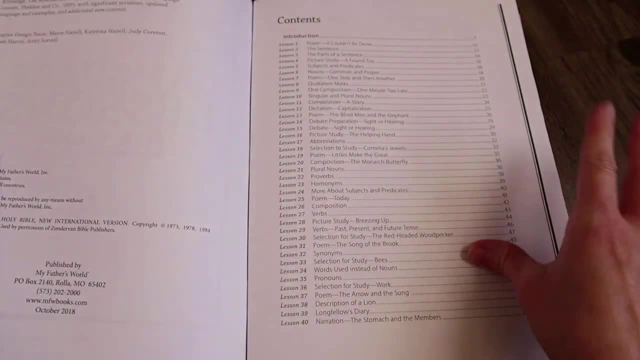 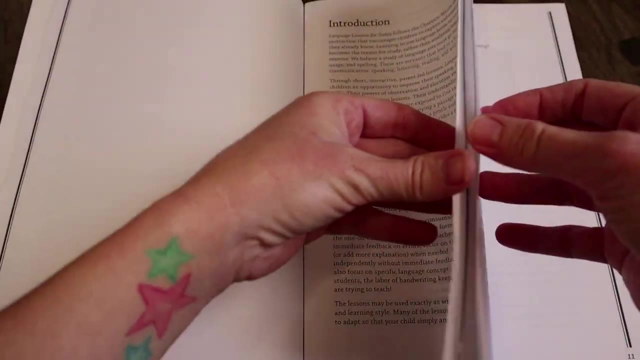 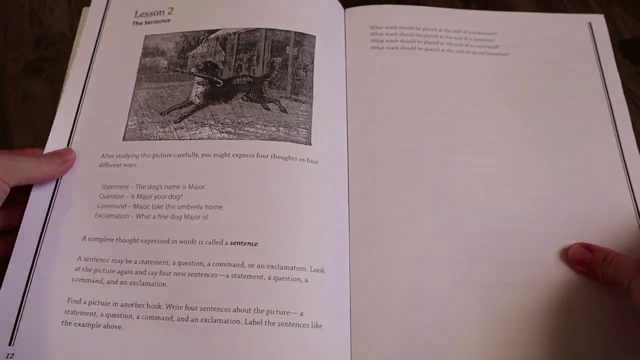 guys so up first is My Father's World Language Lessons for today. Now, if you purchased this curriculum on their website, it is $26.95 and you get a free answer key for each of the lessons. But if you were to purchase it from, say, Christian Book, then the answer key 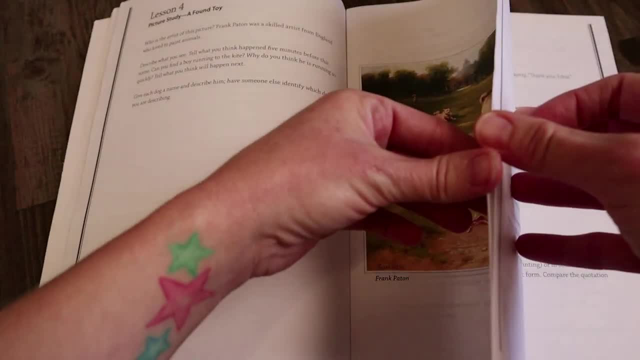 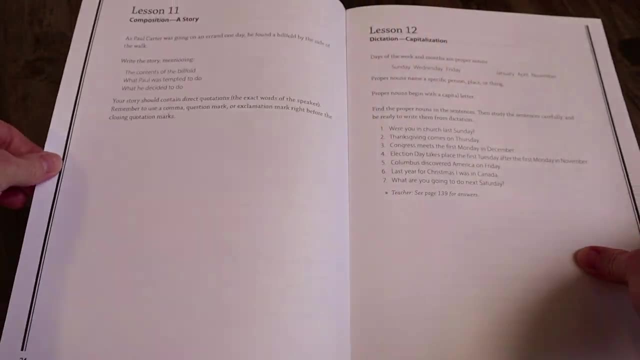 would be $14.95.. So if you were to purchase it from, say, Christian Book, then the answer key would be $14.95.. Now they do have an answer key in the back of the book, but it doesn't cover every lesson, so I'm not sure how much you'd actually need that answer key versus just maybe winging. 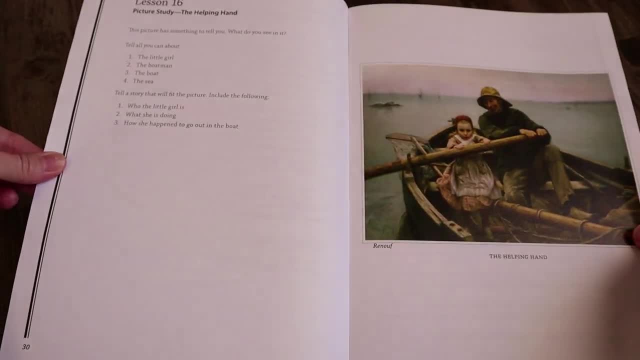 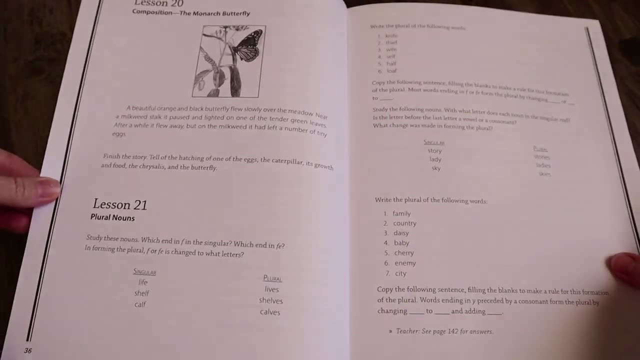 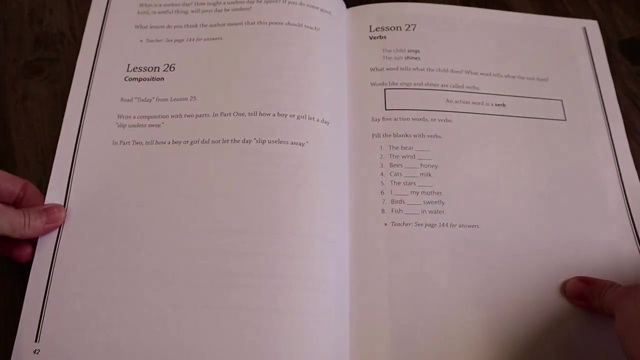 it and seeing how it goes, I'm the wing it type. Now this does take a mix of a classical and Charlotte Mason approach. The really nice thing is it is only three lessons per week. So if you have, if you have other things going on like a co-op or you are getting together with some other, 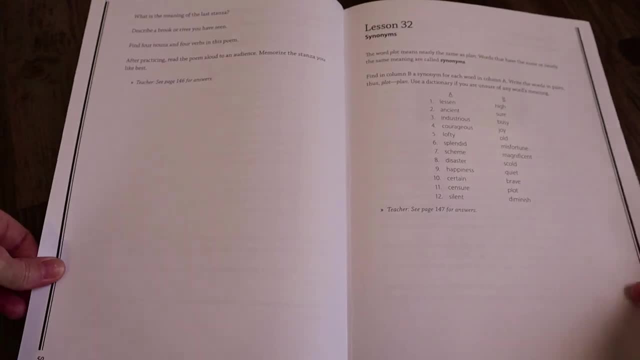 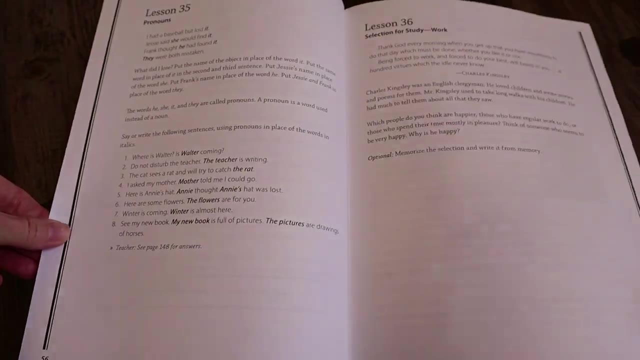 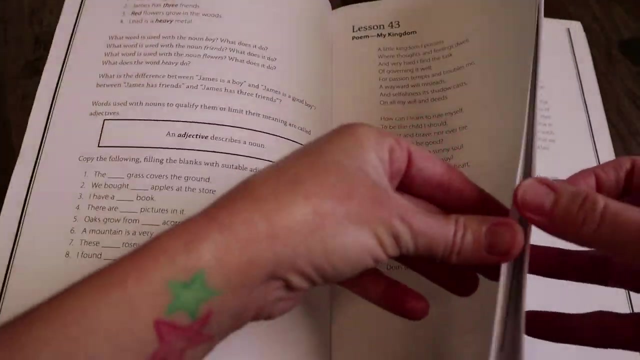 homeschoolers, or you just have a busy life in general, or your child just doesn't, you know, naturally enjoy language arts, then this would be a huge bonus to those of you who are doing those things and maybe just running a little bit of a busier life Each lesson. 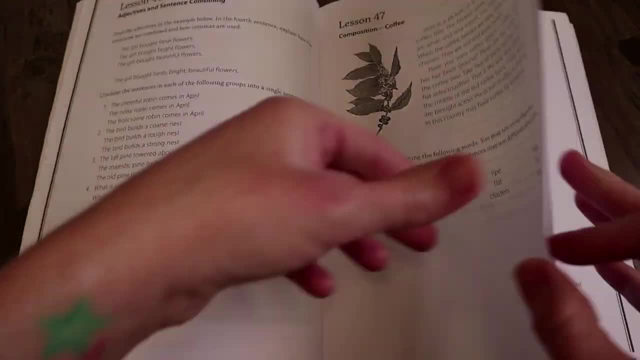 is designed to take about 15 minutes, so it's quick, short, to the point, And then you can just take a little break and then you can go back to your classes. So I'm going to show you some of the lessons that I've learned over the course of the last couple of weeks. 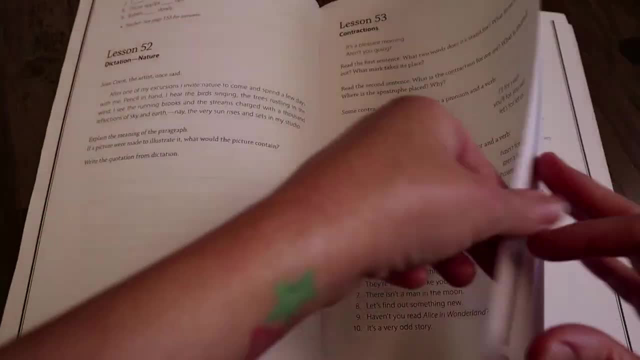 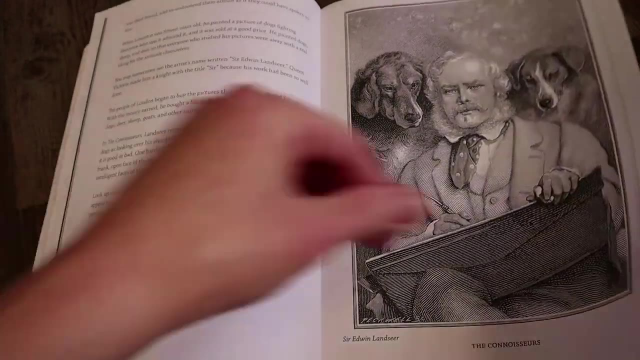 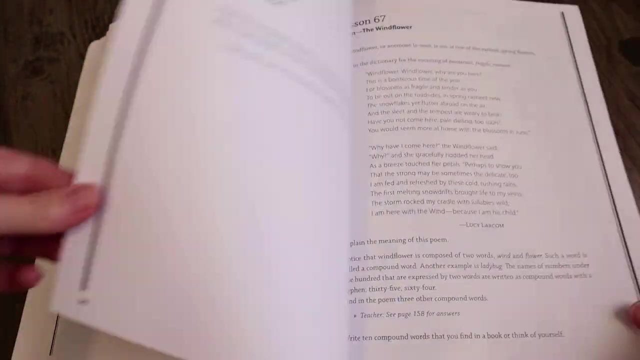 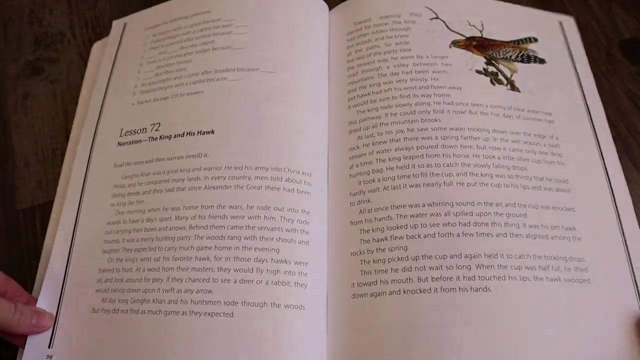 There are about 102 lessons in a year, and some of the lesson types, as you see, will include reading and memorization, some poetry work, picture studies, oral composition, dictation, narration and some copy work. The one thing that I did notice, though, is I didn't really 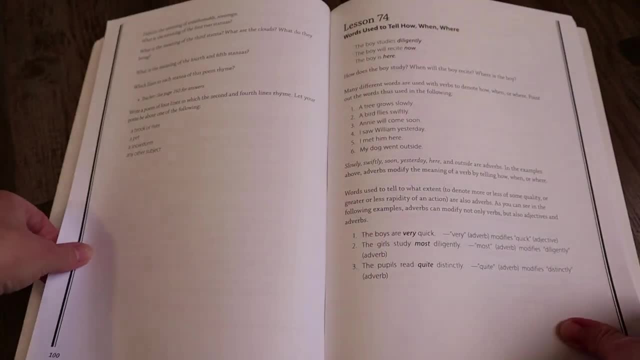 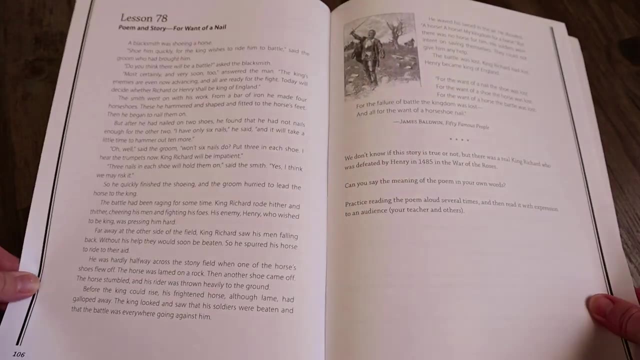 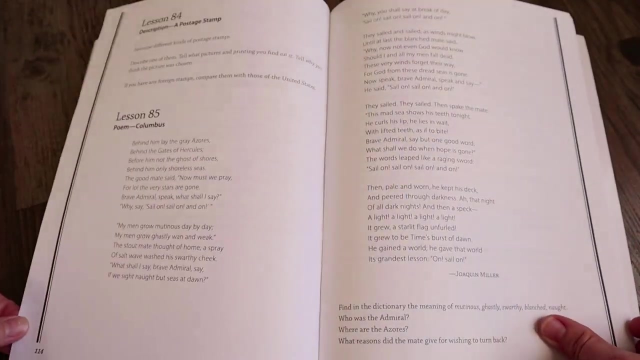 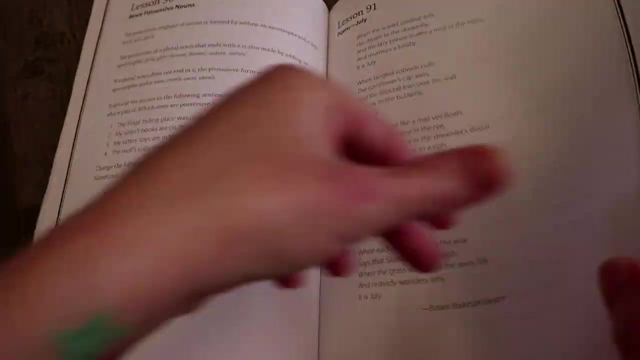 see a lot of spelling work. I would suggest to look into some type of spelling curriculum, or maybe just a spelling workbook for your child's, you know, to meet your child's spelling needs, because I feel like this is lacking in that area. Now, one of the cons is that this is not designed to 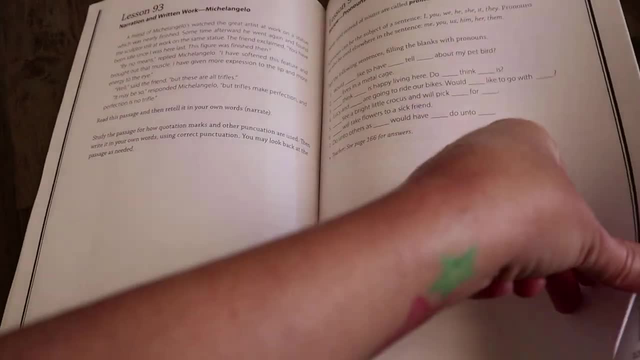 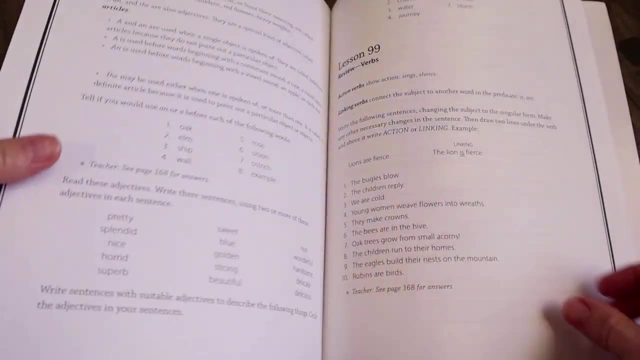 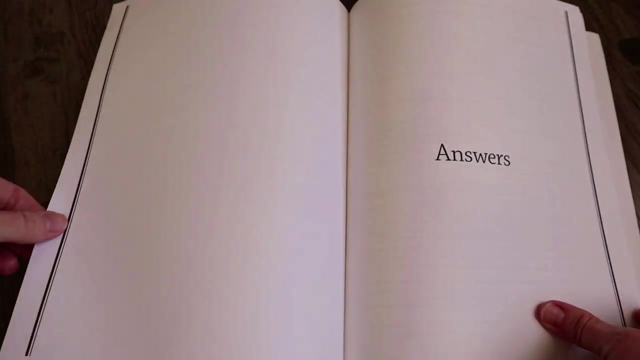 do as independent work it is. it does have a focus on parent interaction, so this is just so you can give your child immediate feedback on errors. So if you are looking for something that encourages a little bit more independence, then that would be the downfall of this curriculum. 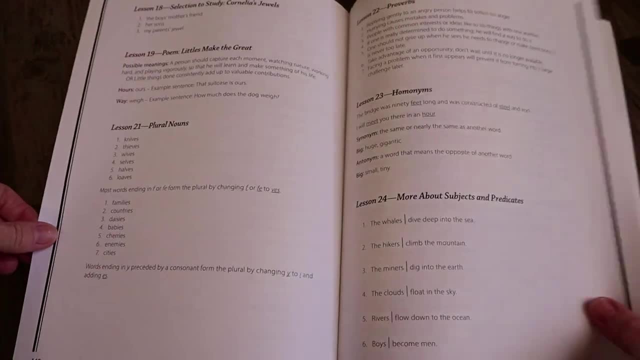 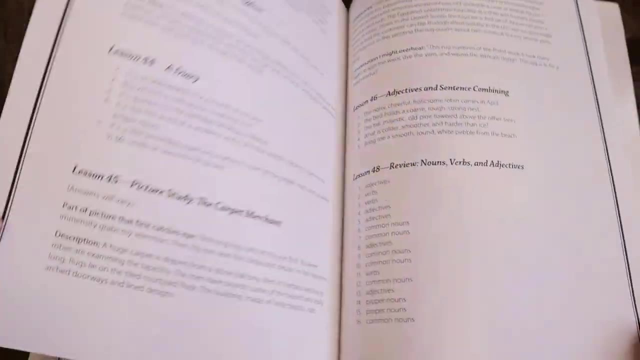 Then you might want to consider another curriculum, but it's also always up to you. I mean, just because they say that this requires parent interaction doesn't always mean that you have to sit there If your child is grasping things pretty well. the first couple: 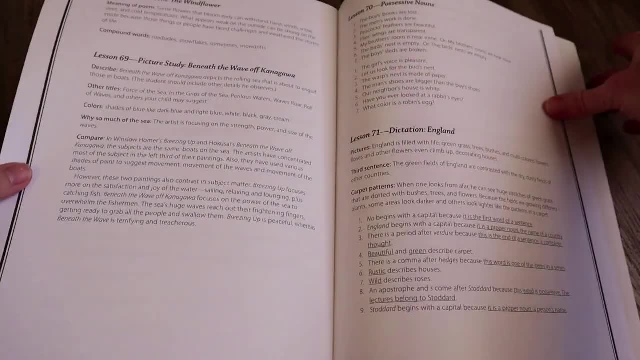 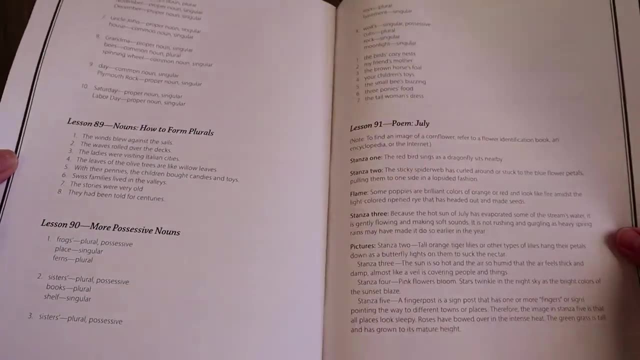 of lessons that you do with them, you'll be able to help them out. So I think that's what them, and you can always give feedback later on. that's just not what the curriculum suggests, so I just wanted to add that another bonus of this curriculum is it is designed to be non-consumable. 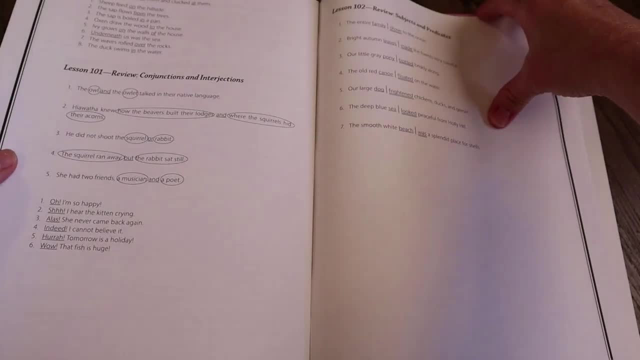 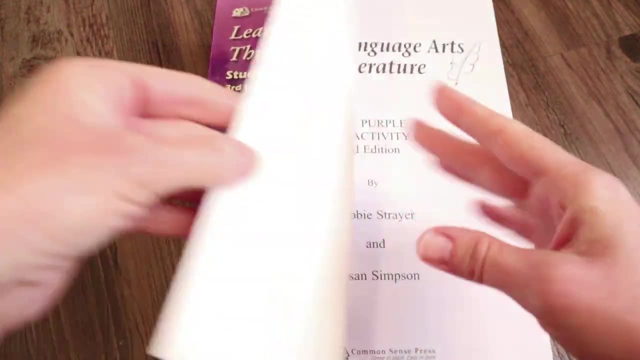 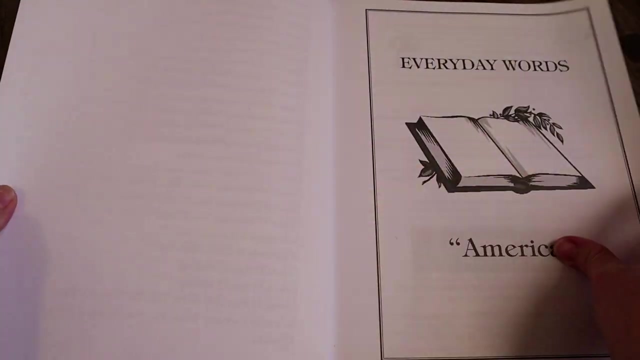 so you can use it over and over with other children and you can also easily resell this all right now for common presses. learning language arts through literature. this is the student activity book. I will give you guys a short flip through of what the teacher guide looks like in. 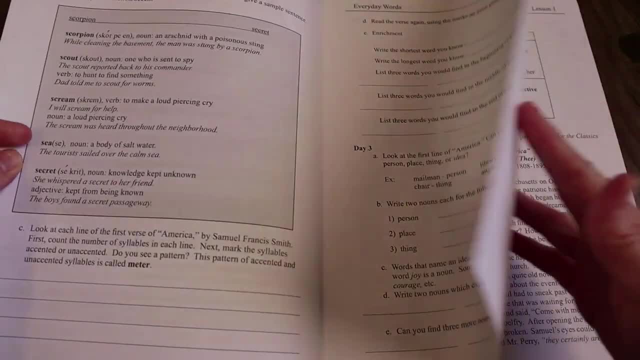 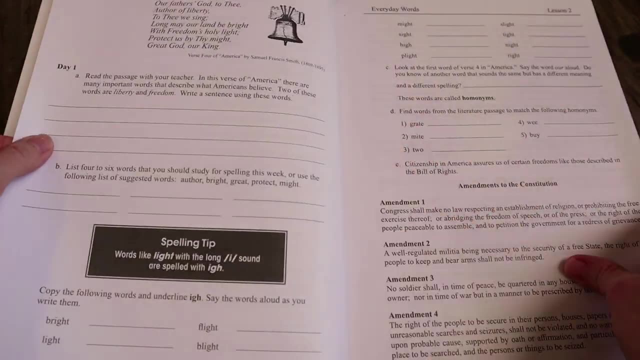 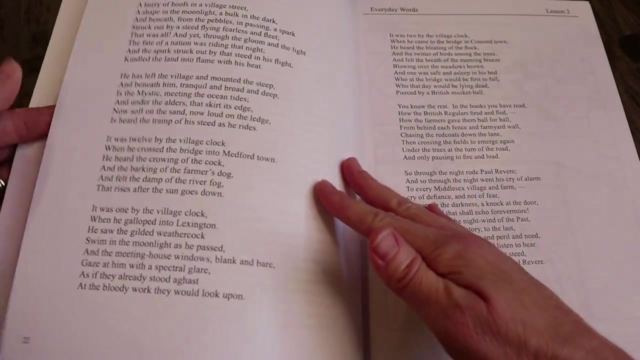 a moment. so here is a recap of all of the lessons that you're going to be doing, the pages that they're on and the book studies that are included. now this on their website is $28 for the student book and $34 for the teacher book. like I mentioned, you can also purchase this on christianbookcom. 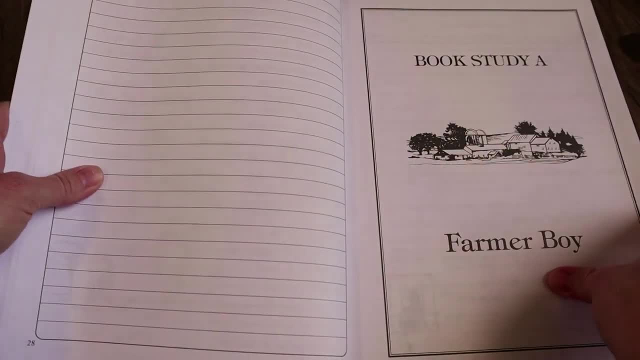 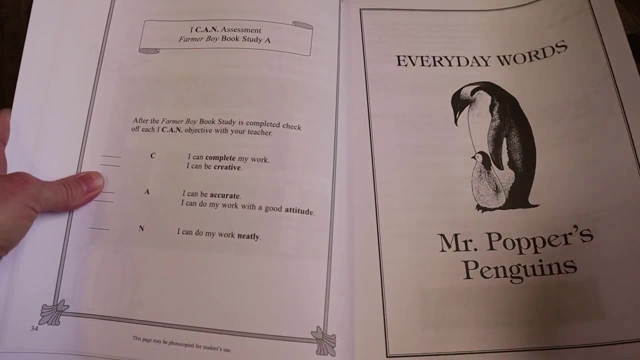 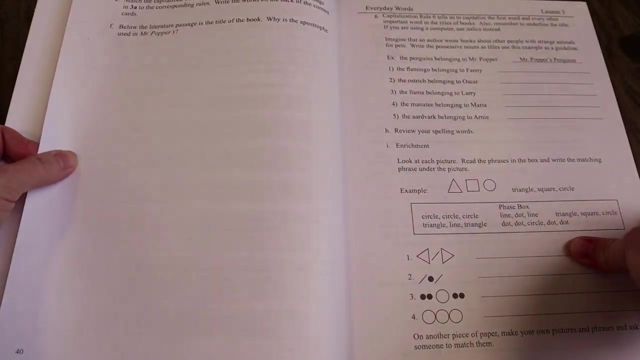 I believe I I I got both of these and I believe I did it through during one of their promotional sales where they gave you an extra percent off. so I want to say I paid about $65 for both curriculums to include the teacher set, so it was fairly inexpensive altogether. now this has an integrated language. 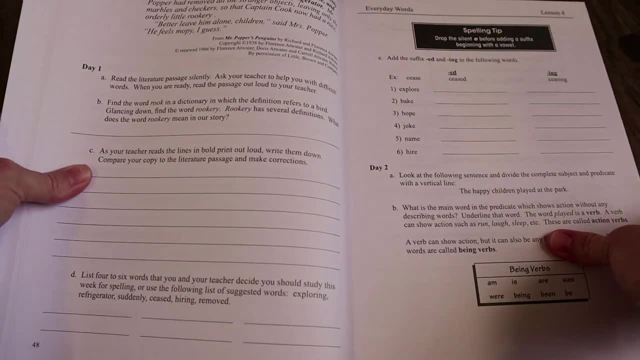 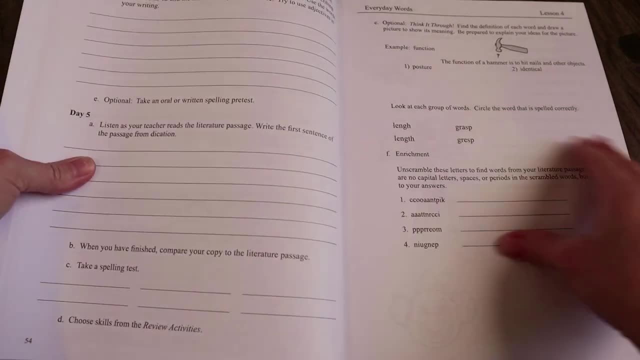 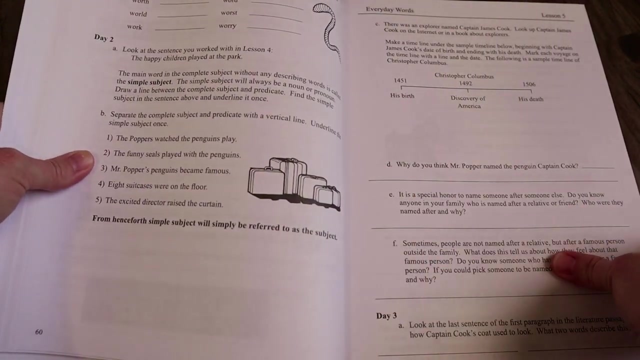 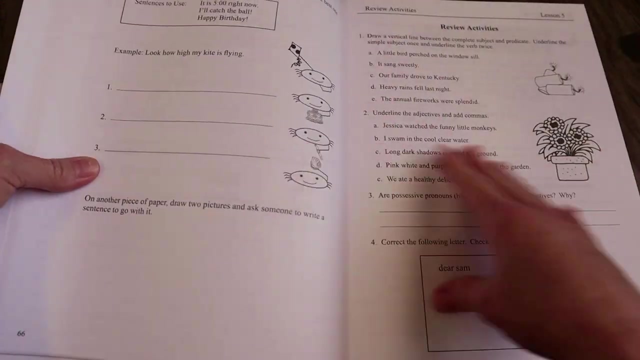 approach. it is five days per week, which concludes basically one of the lessons, and there's a total of 36 lessons, so it's a full, traditional one-year curriculum. it also includes four book studies within the lessons and most curriculums will tell you how many minutes it. 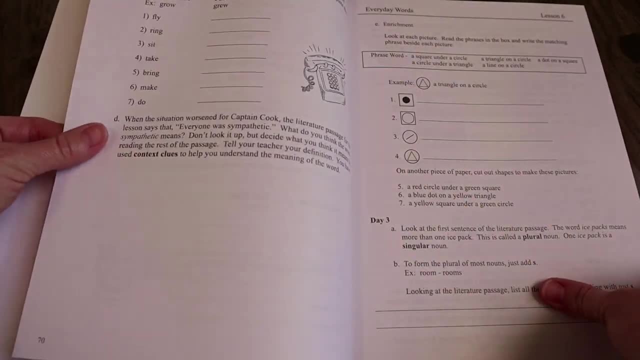 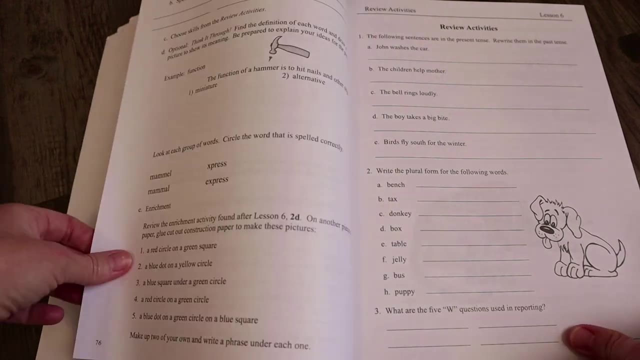 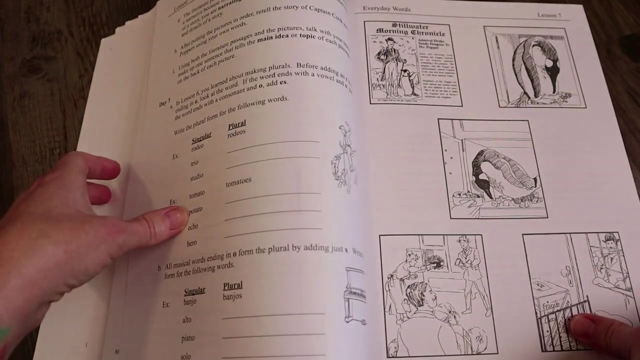 should take your child roughly, just like an estimated time frame. I did not see that mentioned in either the student book or the teacher guide, but just looking at these lessons, depending on your child and how much they they love or just like language arts, and just how fast. 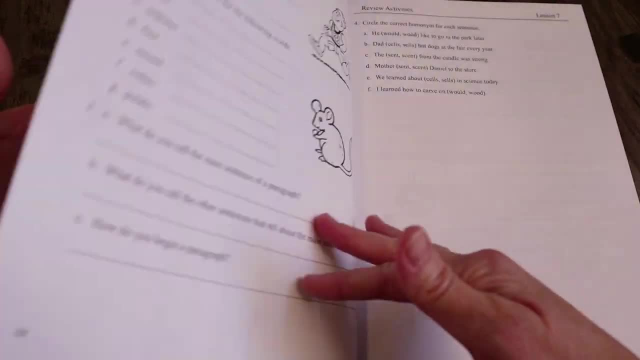 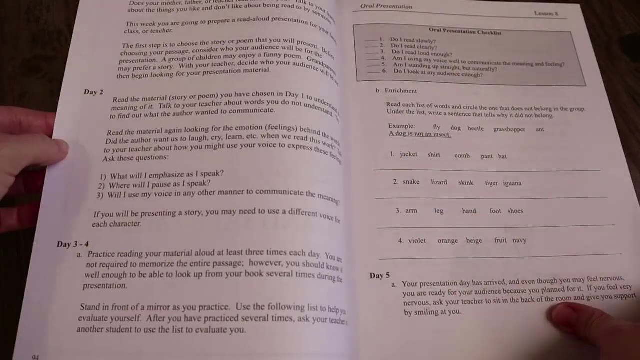 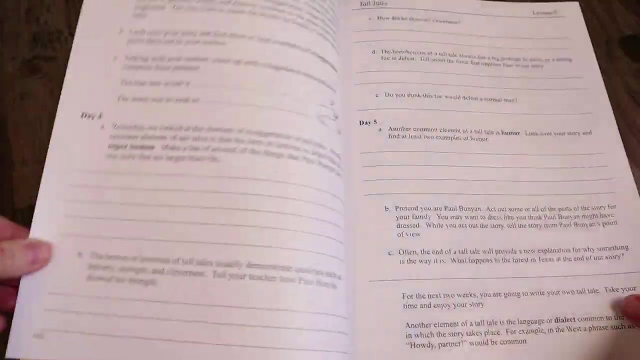 they work through it and understand concepts. I would estimate that this could take anywhere between 20, maybe 30 minutes to 45 minutes, so it does take a little bit longer than the my father's world, but probably also right on pair with or right on par with, like something like the good. 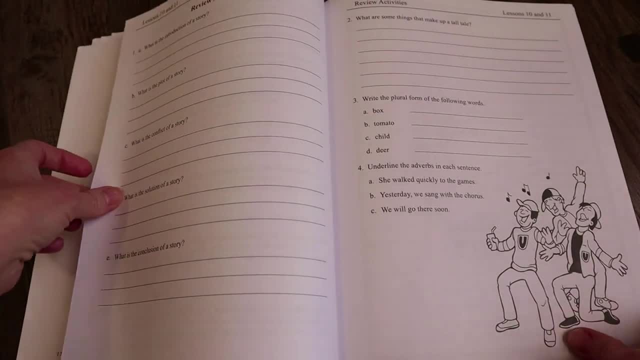 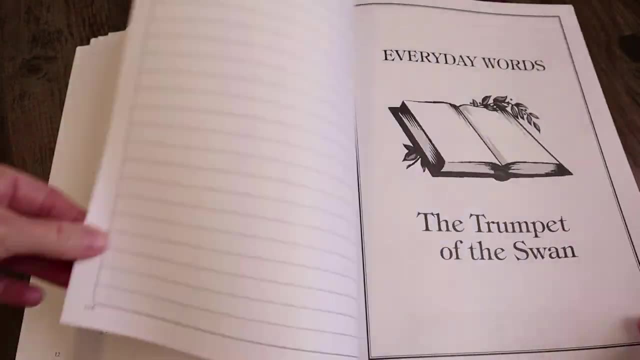 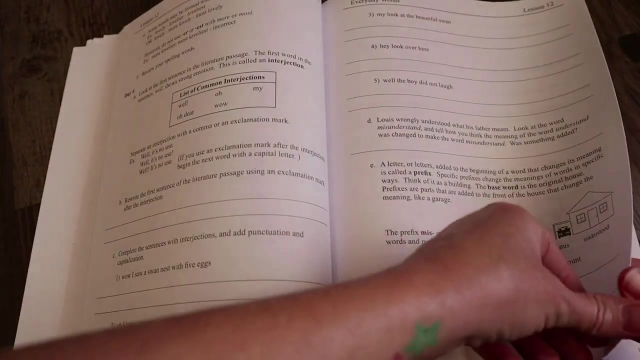 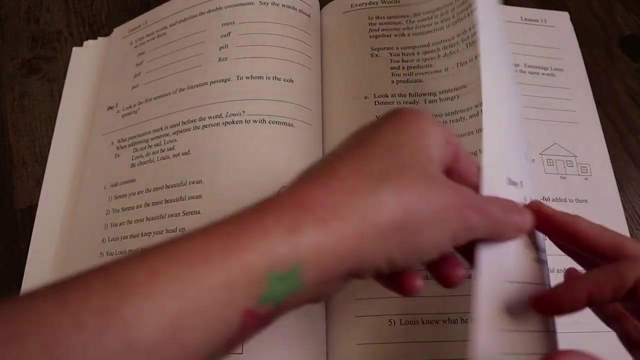 and the beautiful, if you guys have used that. now this comes with, like I mentioned, the student activity book and the teacher book. so you will need the teacher book for all of the answers and just the breakdown of the lessons. and a day looks like you listen to the literature passage, so you're sitting down and you're reading it with 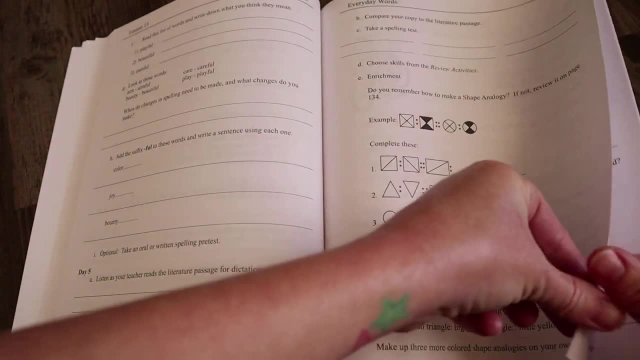 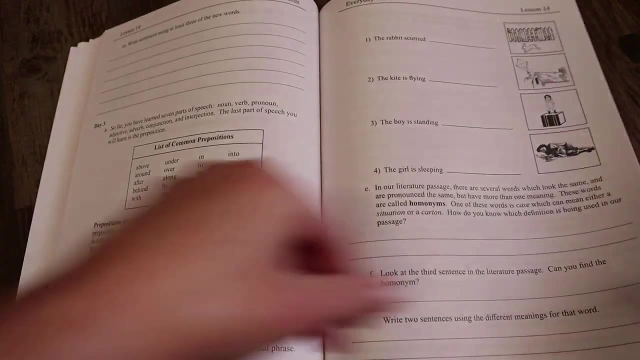 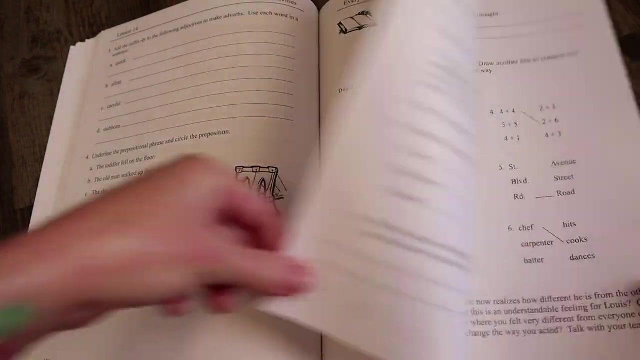 your child and then you use a dictionary or your child uses the dictionary. they will choose spelling words to work on, you'll have a discussion, they'll be given a description of something that the lesson is going over and they'll make a list. now, uh, there are four. book. 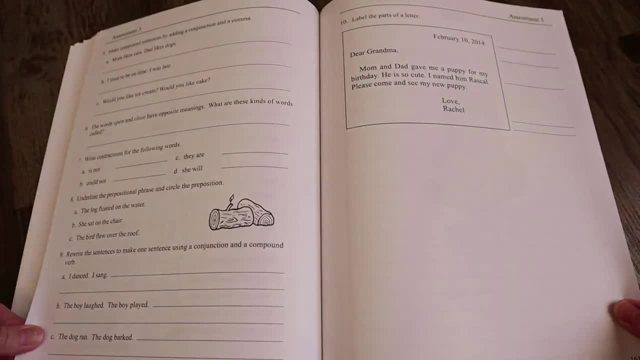 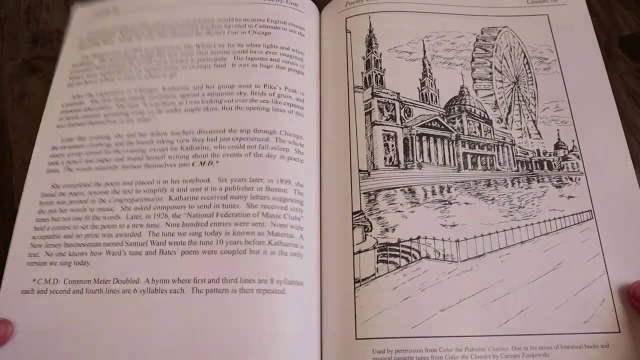 studies in this curriculum. one of them is a book study on a book called number the stars. that is a story about a young girl who was living in Germany during the time of Nazis, so and it just kind of goes over her life, and she's living in Germany, and she's living in Germany, and she's living in. 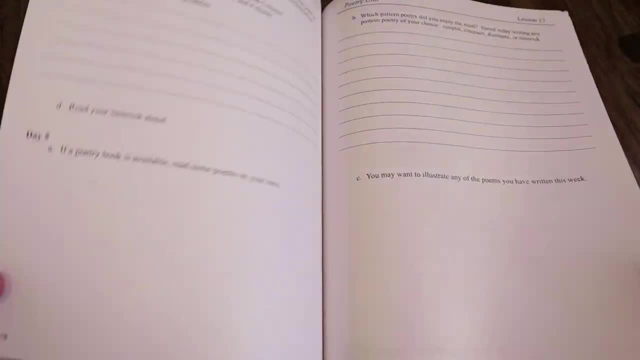 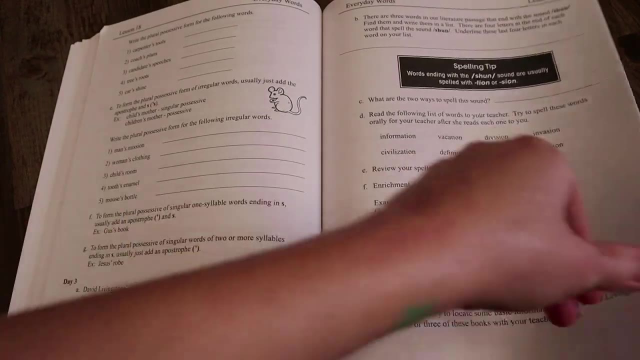 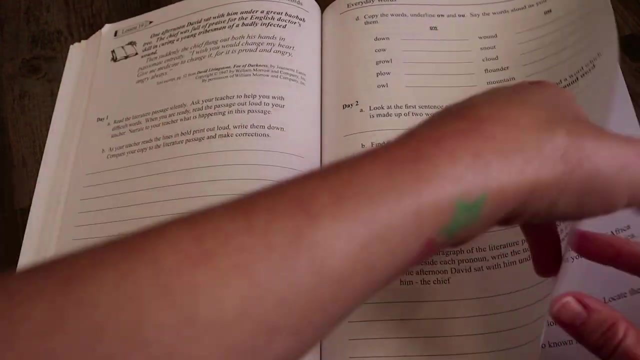 how it's altered from all of the hardships that were going on during that time. so if your child is a bit sensitive and you're not quite ready to introduce that topic, I just wanted to mention that, as you know, you might want to consider skipping that book or replacing it with a 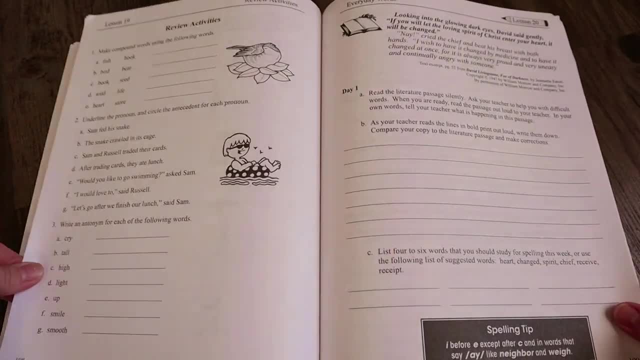 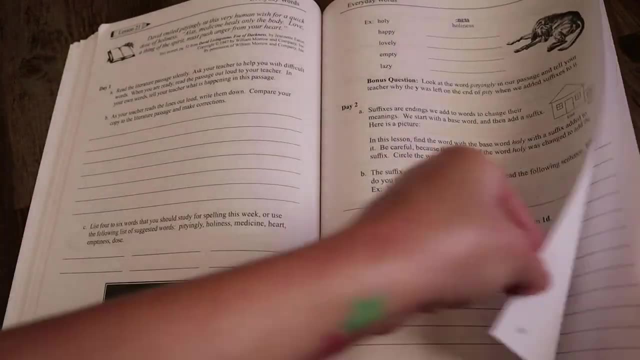 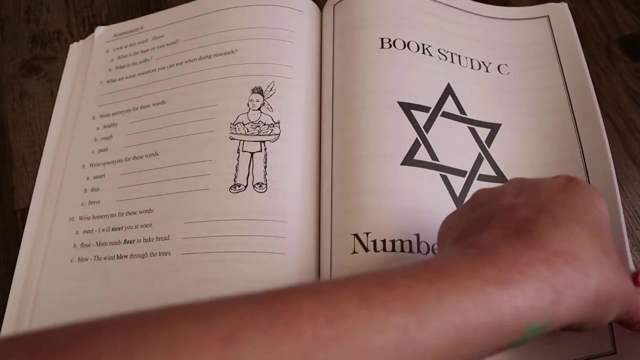 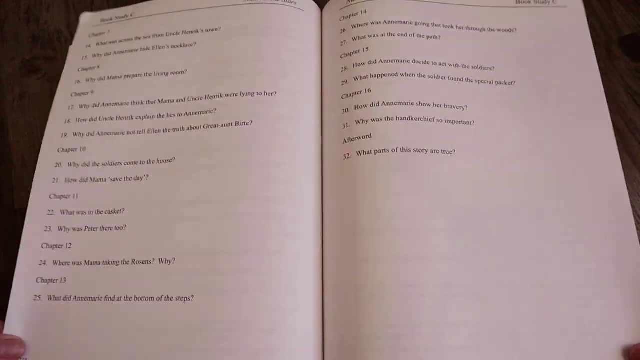 different book study from either another company or one that you come up with. the other remaining studies are a farmer boy, the trumpet and the Swan and Katie woodlawn, and then, at the very end, I'll go back and I'll show you a little bit more in depth on what a 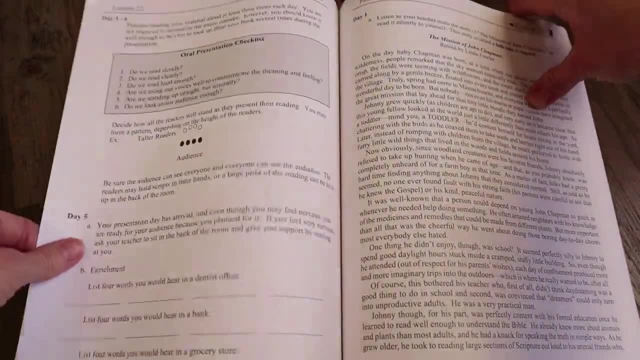 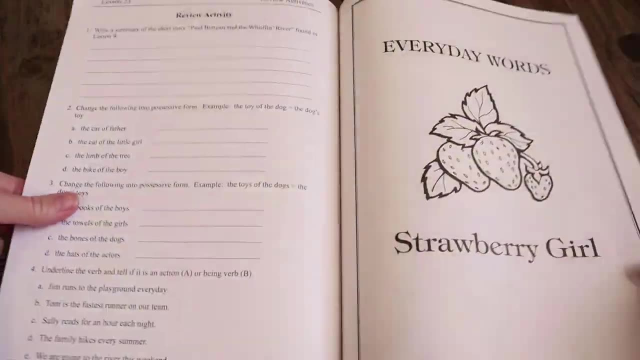 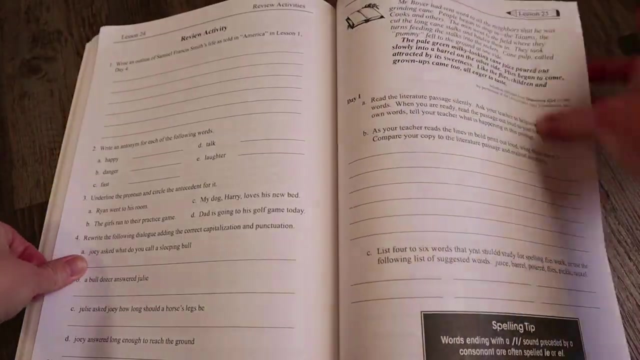 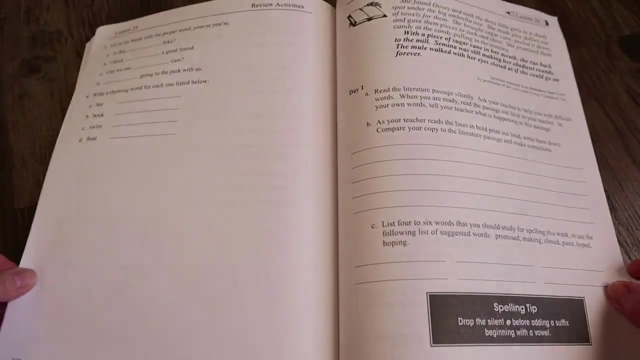 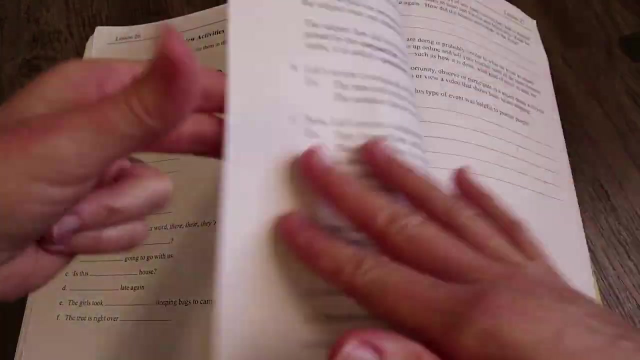 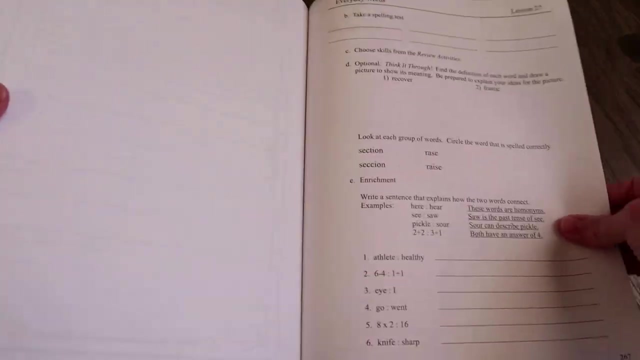 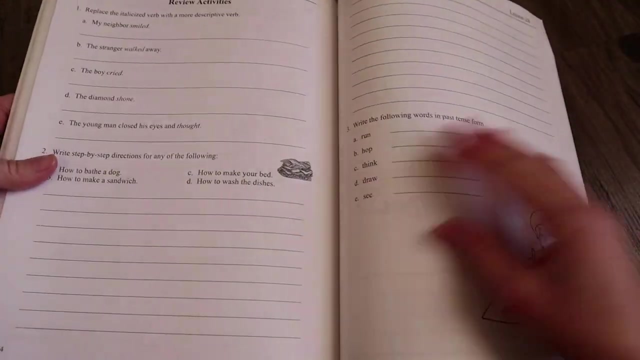 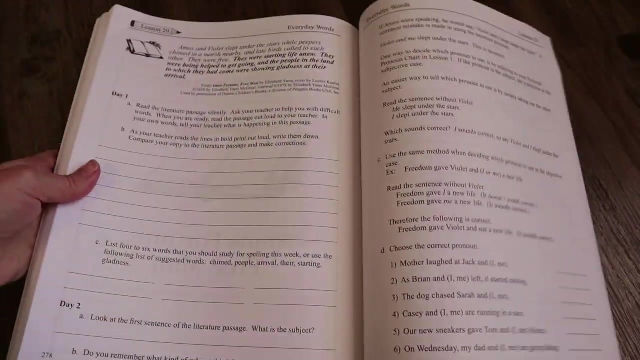 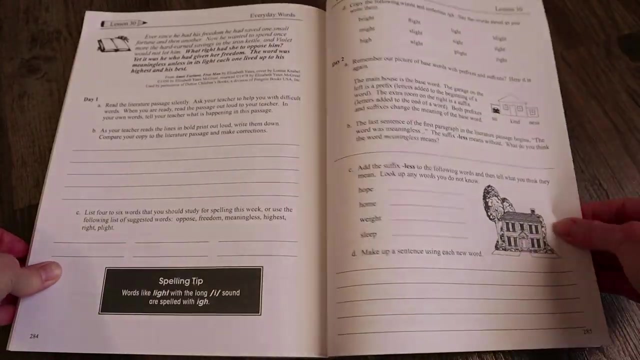 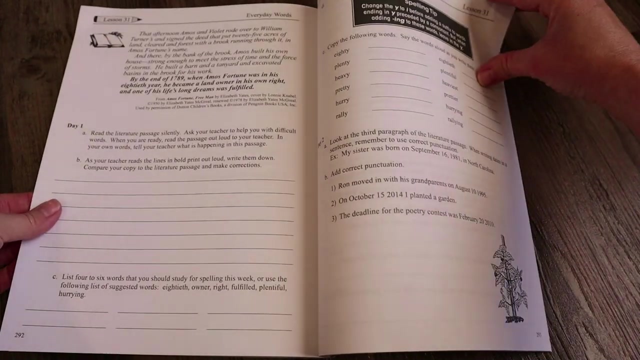 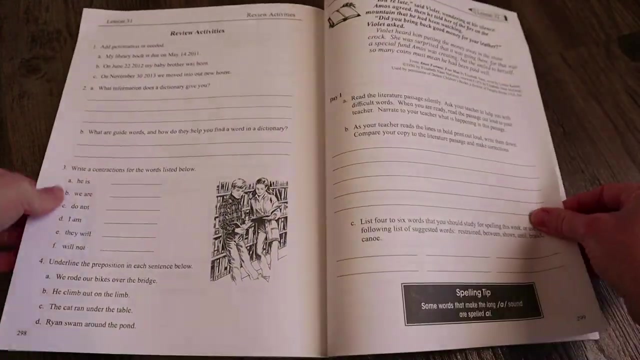 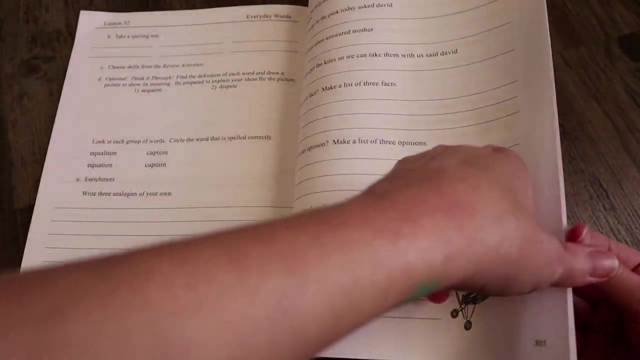 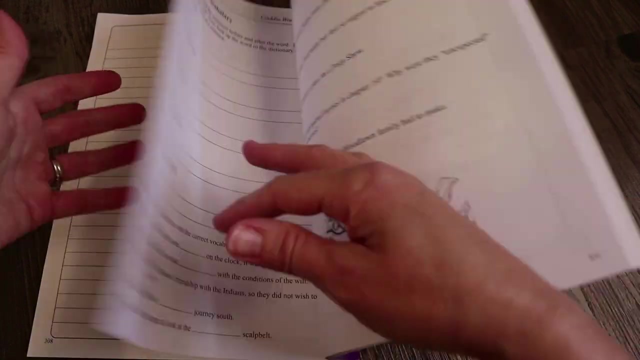 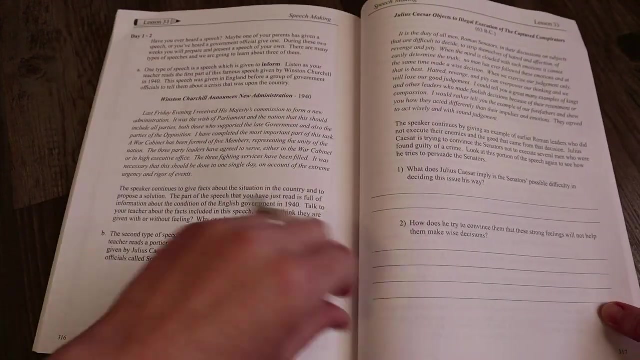 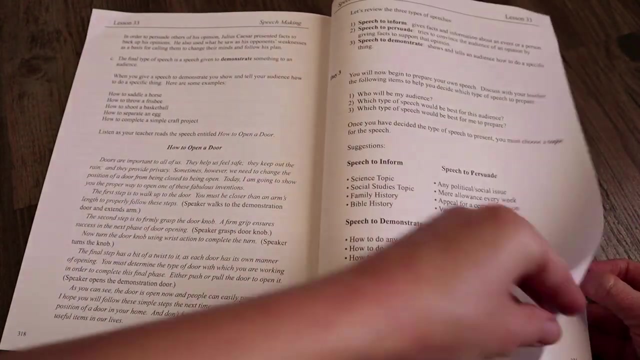 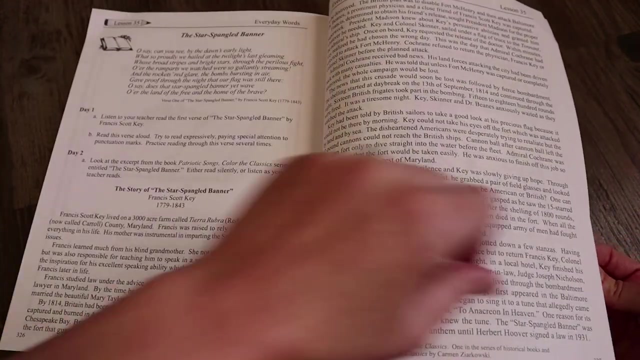 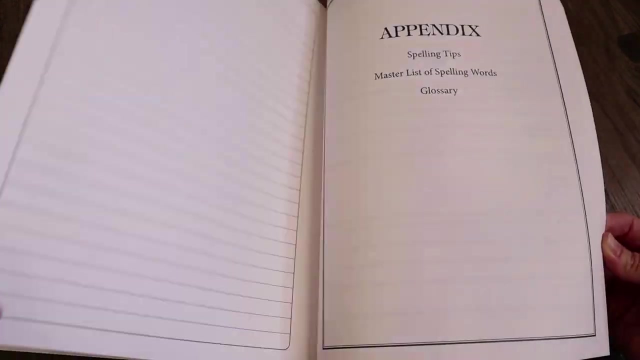 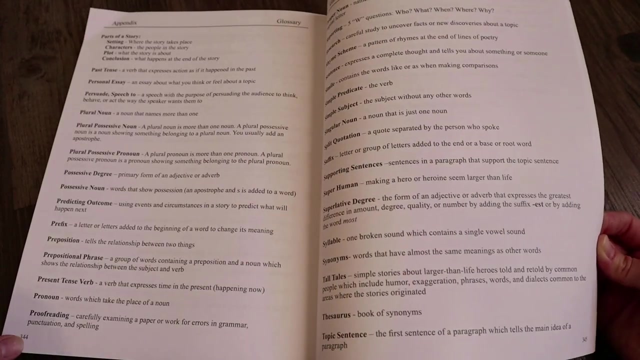 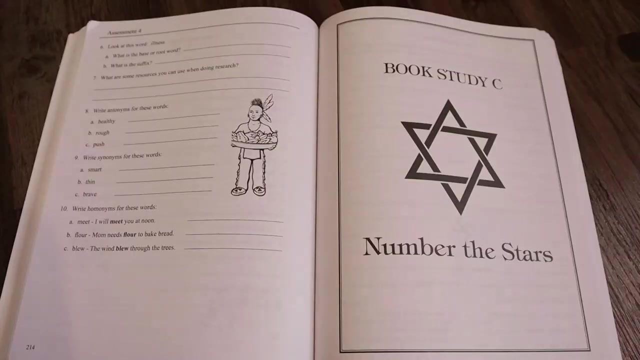 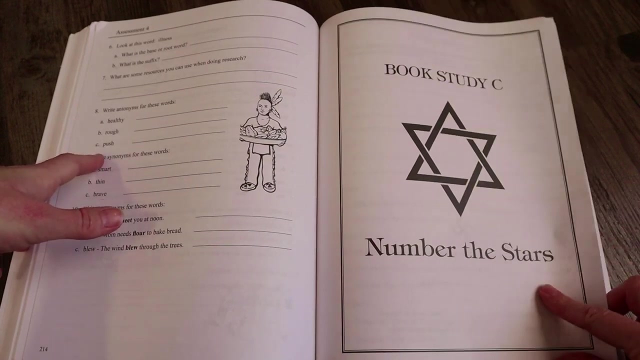 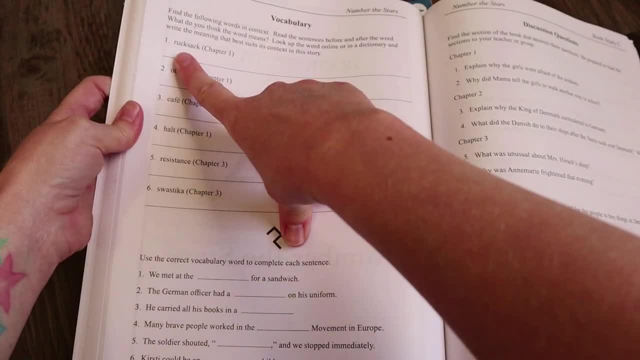 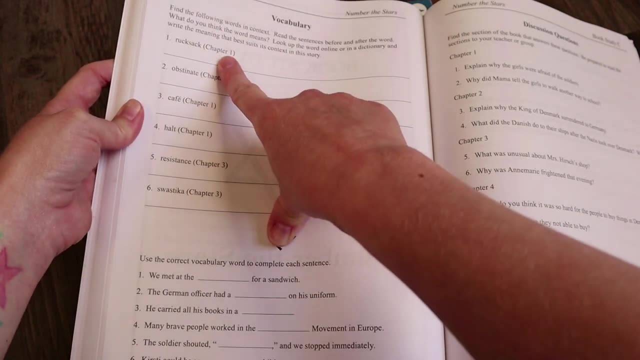 So it starts with vocabulary and the child is gonna be encouraged to go get their dictionary to look up what each word is and write the description. It gives them the chapter that that word is mentioned in And then they're gonna use the correct vocabulary word. 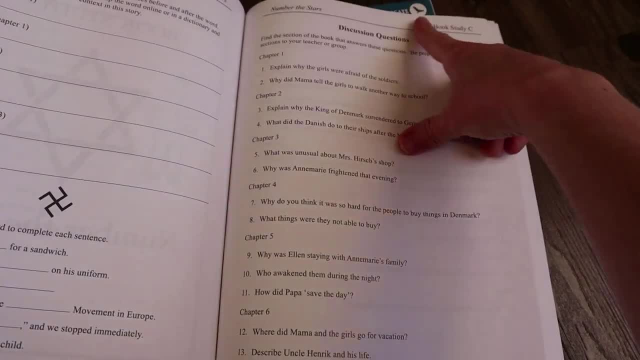 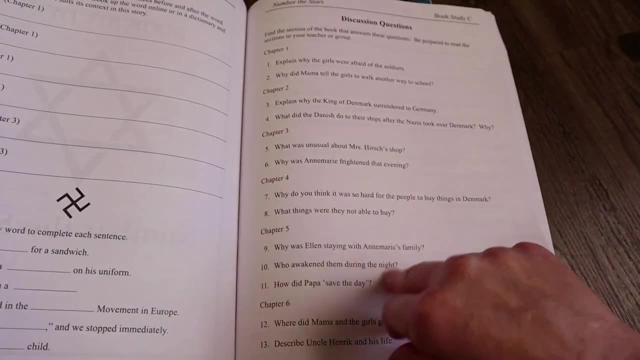 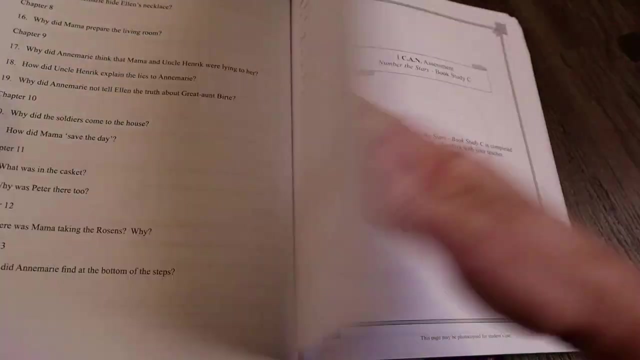 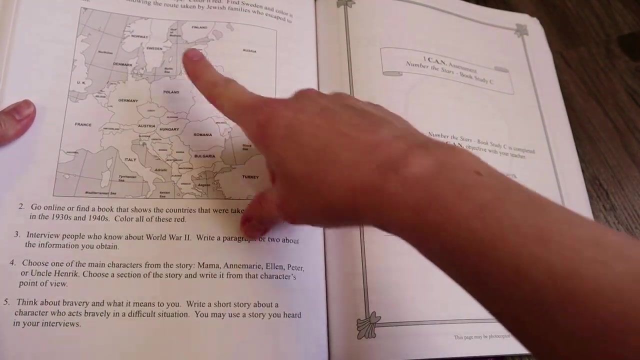 to complete each sentence. On the following page there is some discussion questions for each chapter of the book. That continues on to the following pages And then there are some story activities where your child will be encouraged to go and look at the map and locate Denmark on the map of Europe. 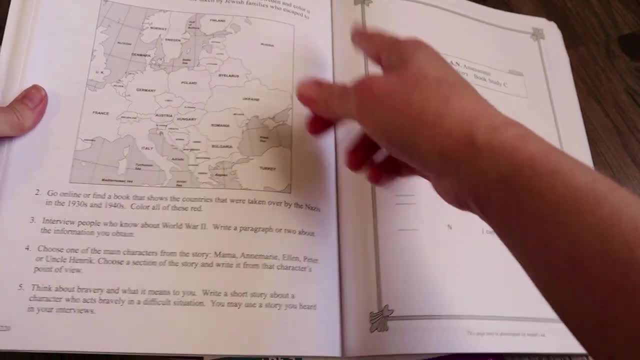 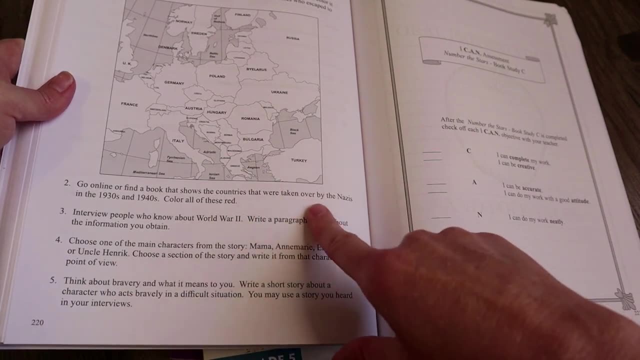 color it red, find Sweden, color it green, and so on and so forth, And then you're gonna have your child go online and find a book that shows the countries that were taken over by the Nazis in 1930s and 1940s. 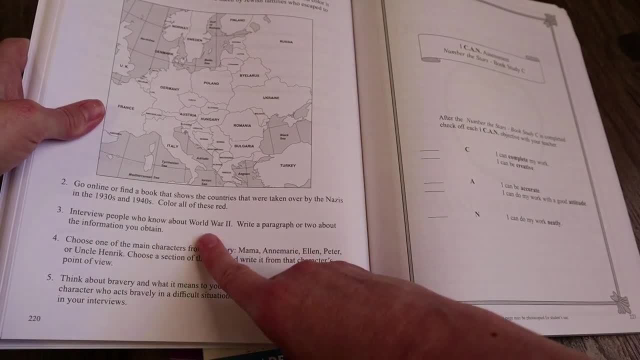 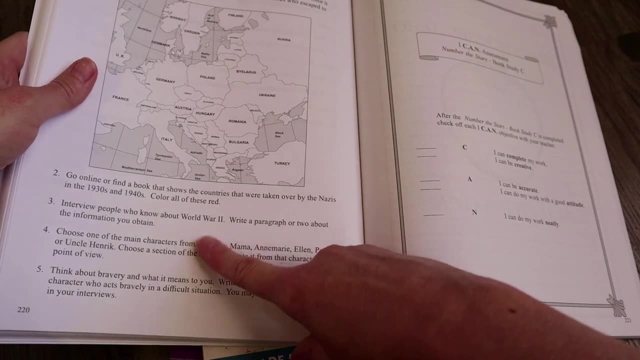 color, all of those red- interview people who know about World War II, write a paragraph or two about the information you obtain. So I mean, even if you don't know anybody personally, you can even look up a documentary where people talk about it and have them write on that. 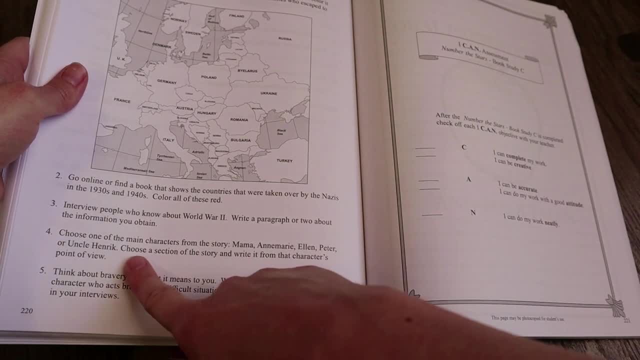 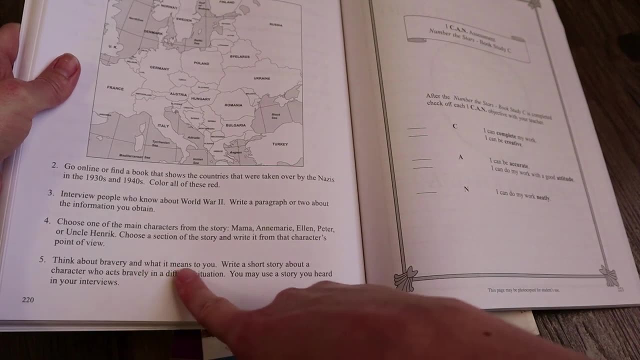 Choose one of the main characters from the story and then have choose a section of the story and write it from that character's point of view. Think about bravery and what it meant to you. Write a story about a character who acts bravely in a difficult situation. 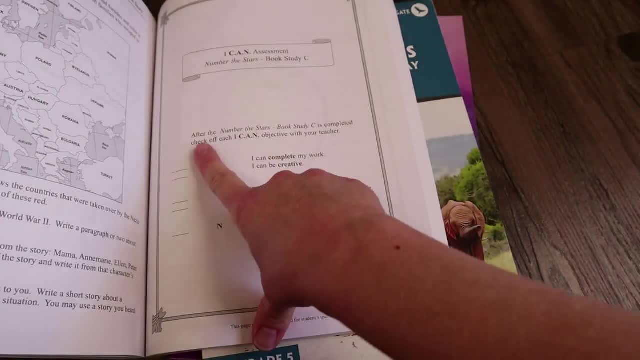 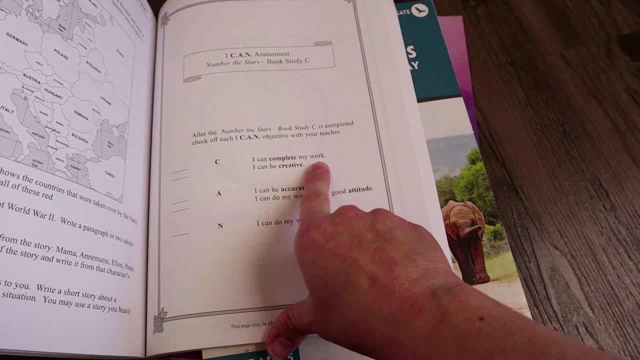 And then it ends with just an assessment, saying, once it's completed, have your child check off the I can objective with you. So it says: I can complete my work, I can be creative for C, For A, I can be accurate. 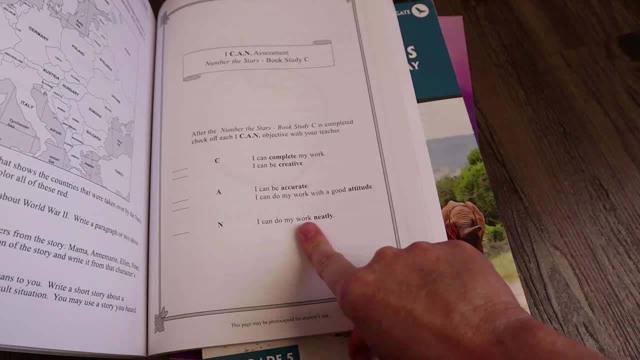 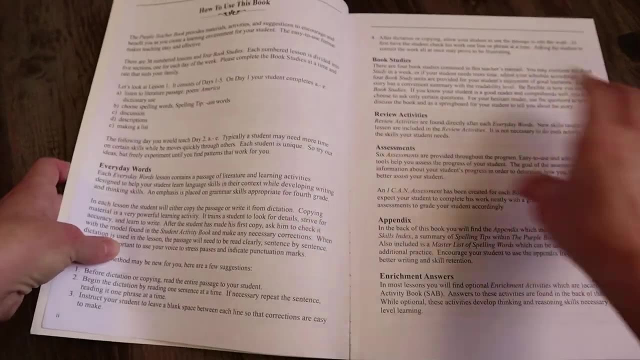 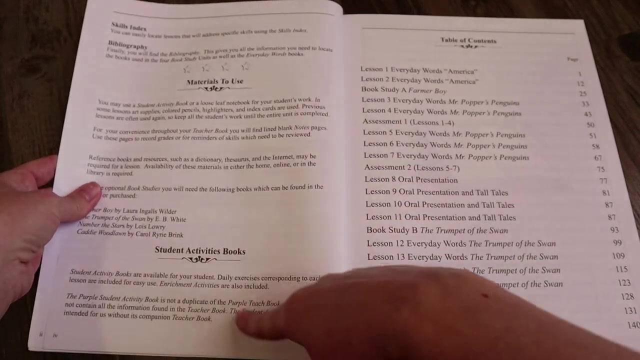 I can do my work with a good attitude And N I can do my work neatly. Okay, and then just a quick look into the teacher book. So it just gives you basically a how to use this book. little intro materials that you'll need. 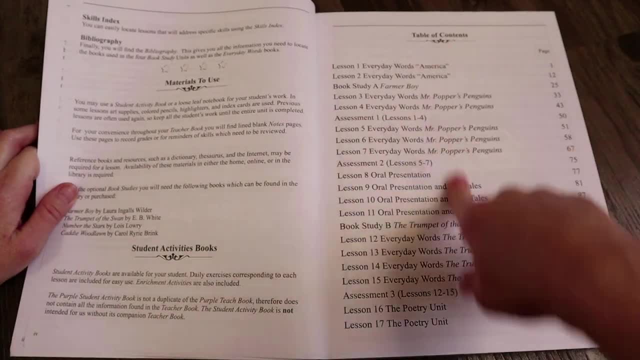 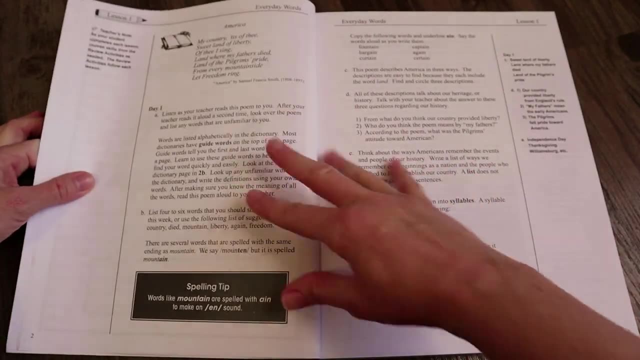 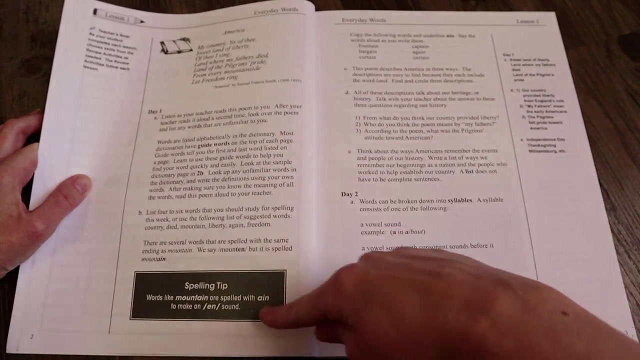 student activity books that are required the same table of contents that you got in the student book, And then each page will look similar to what your child's book looks like In terms of what their lessons are, And then on the side, it will give you the answers. 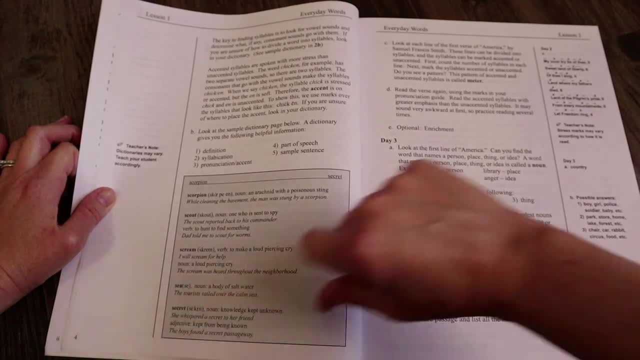 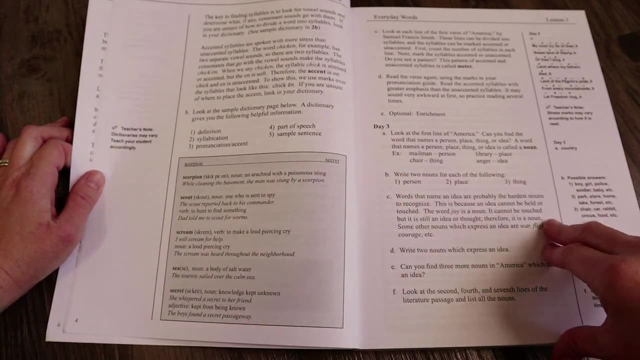 And then it also has a side on the page where you can also make your own separate notes. So it's nice because even for like the dictionary terms they fill it in for you, So you're not having to go and double check your child. 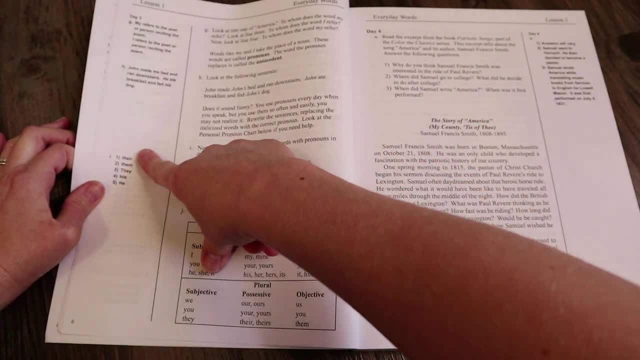 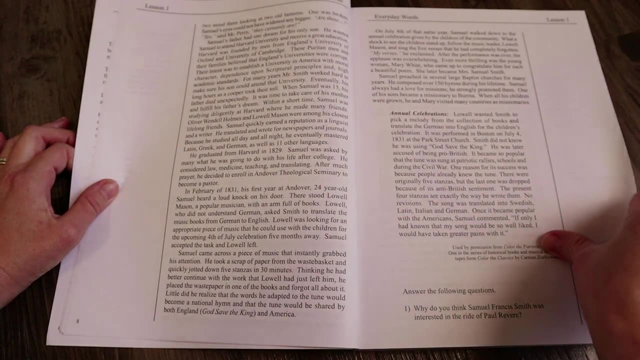 and what they wrote down, And then again they have the answers on the sides for any questions that they have. Okay, So that's what you have within the lesson, All right, So now I'm gonna post the comparison chart for you guys. 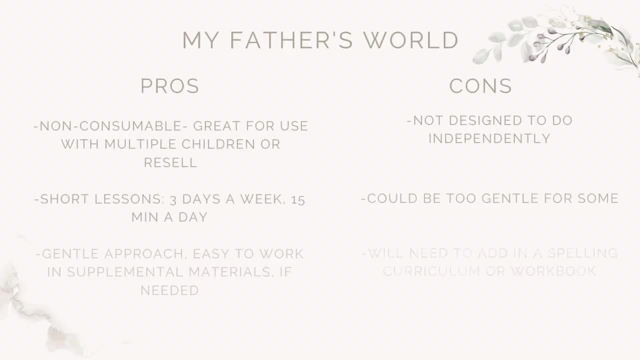 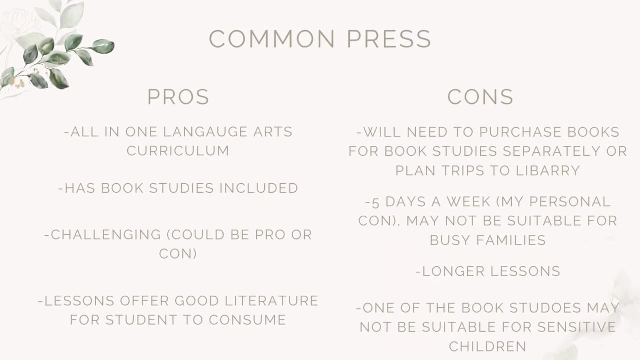 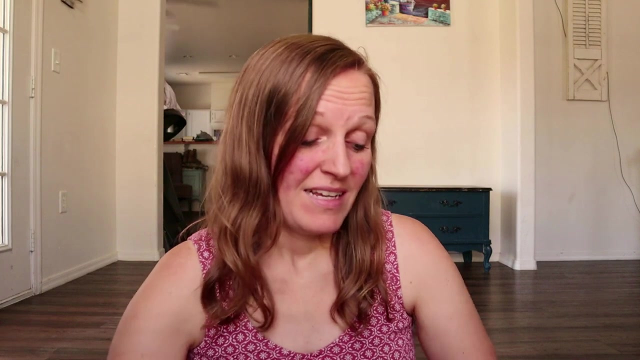 and then turn around the camera. All right, you guys. So that is it for the flip through. I hope that this helps seeing inside the books and just helping you to make your decisions for the upcoming year. I know it can be so hard to find. 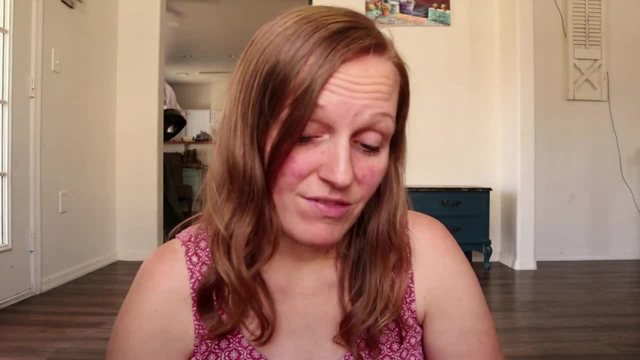 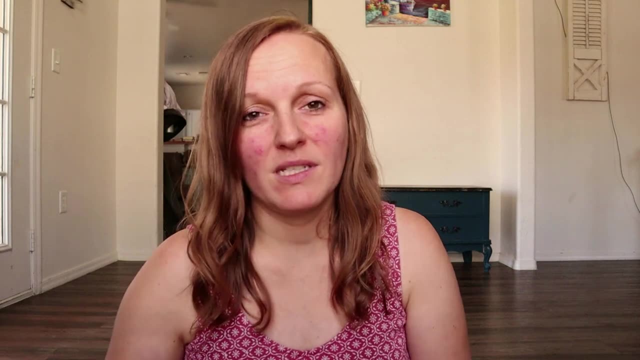 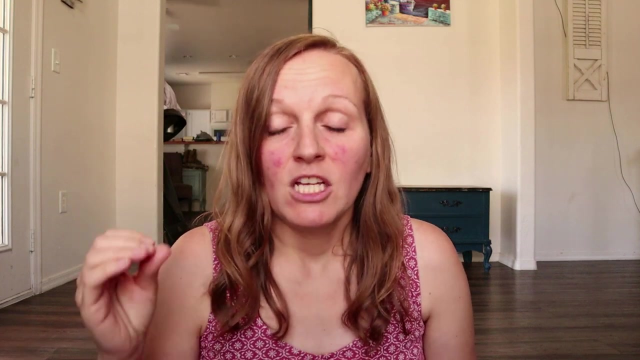 a good language arts curriculum. One of the beautiful pieces of advice that I heard recently on a podcast was to not always just focus on your kids having good grades in everything or doing well in every subject, but to instead focus on their strengths and the curriculums and the subjects. 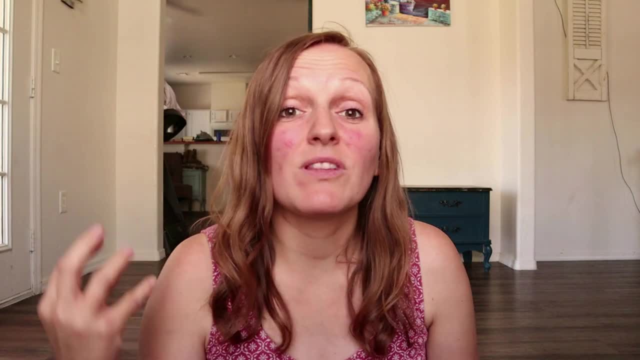 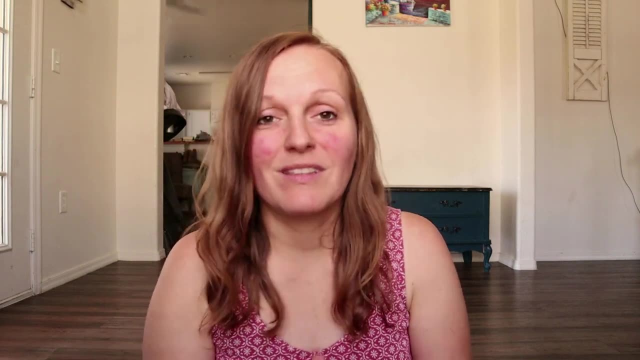 that they really thrive in, Because that's where their strength is, That's where their passion is. So focus on those things and don't necessarily put so much weight and pressure on the things that they don't do so well- And not to say that they can't get better in those things. 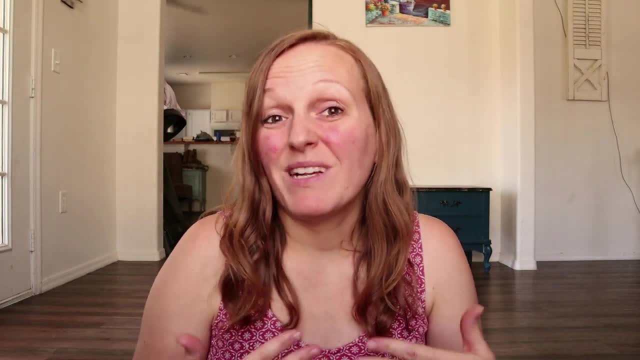 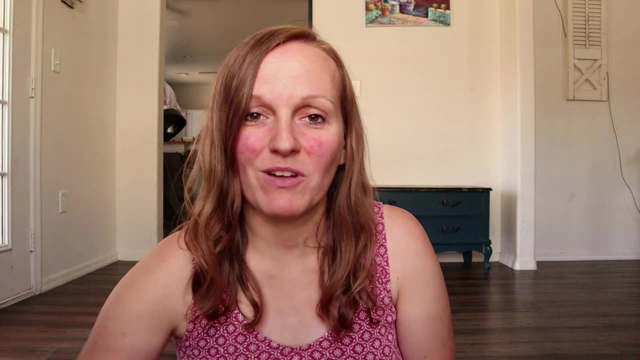 but if they're weak in those areas, it might just be because they don't have a joy for them, And so you just driving it in even deeper is going to kind of push them away from the very thing that you're trying to bring them to. 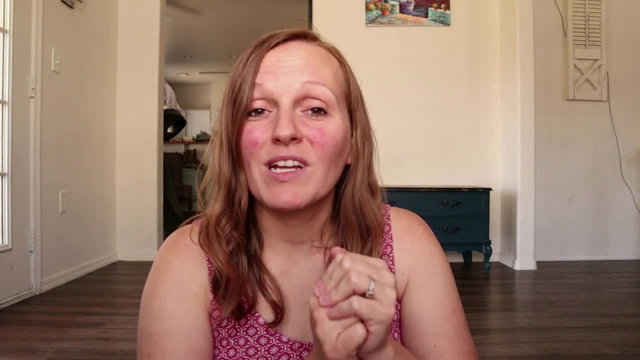 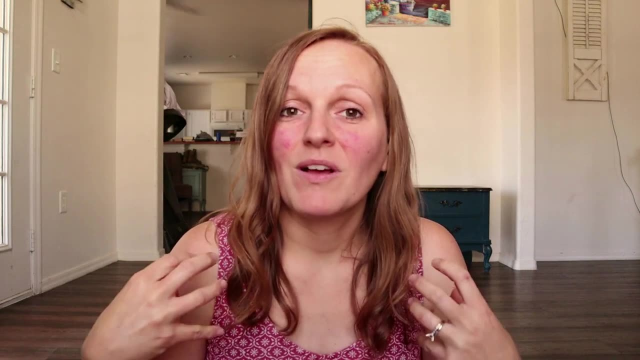 So hopefully that tip can help you guys Also: don't freak out while you're choosing curriculums. I know that, like you know, as we get even more into the summertime, instead of relaxing, some of us are thinking like: 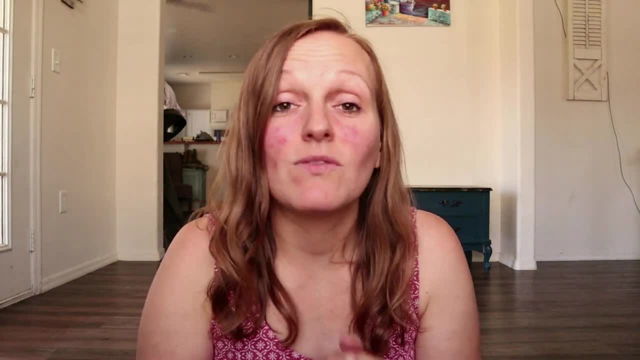 oh man, I still don't even know what I'm using for this subject, And that can be very stressful. but breathe, mama, because it's not that big of a deal. You're not like I said before, you're not going to be on your deathbed. 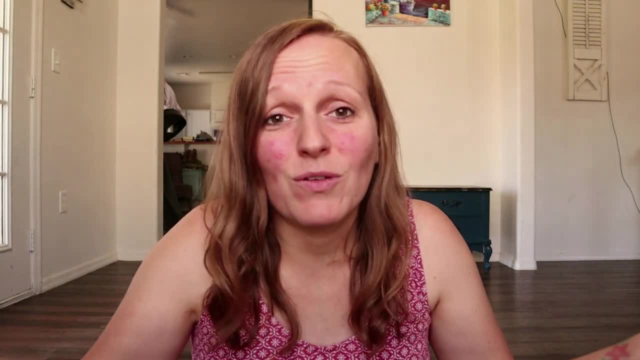 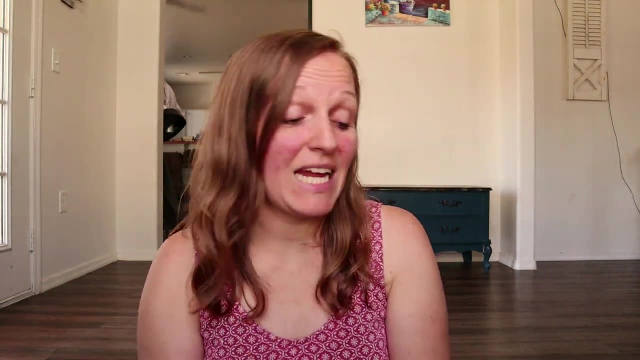 or like 90 years old thinking man. I wish I would have chosen a different math curriculum for little Johnny. It's not going to matter. So while it feels like this huge decision today, it's not going to be make or break in the long run. 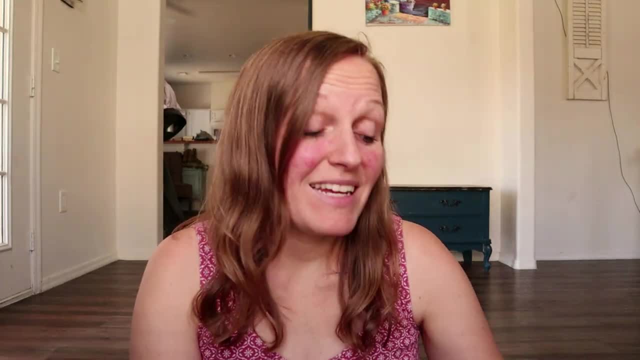 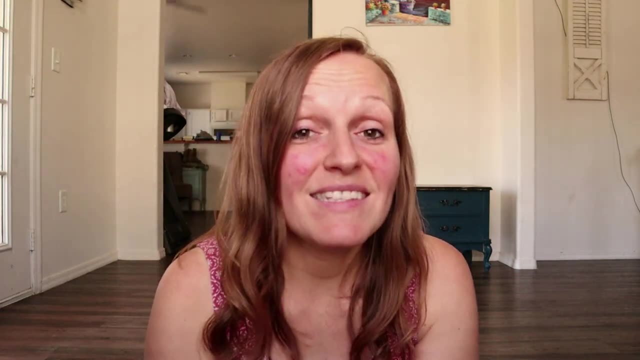 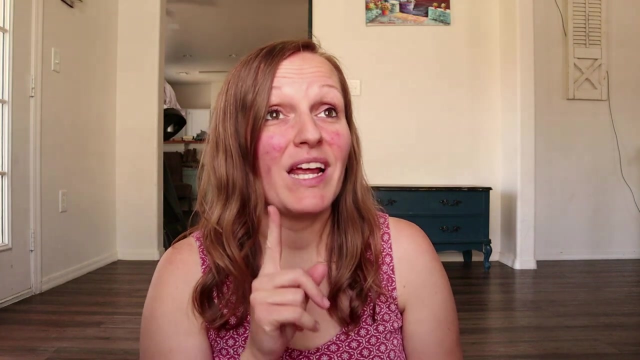 So just focus on doing your best. I hope that seeing the whole flip through of the books was helpful to you guys in making your decision. I will have tons of curriculum reviews and flip throughs coming up for you guys. I actually got my hands on a fifth grade.